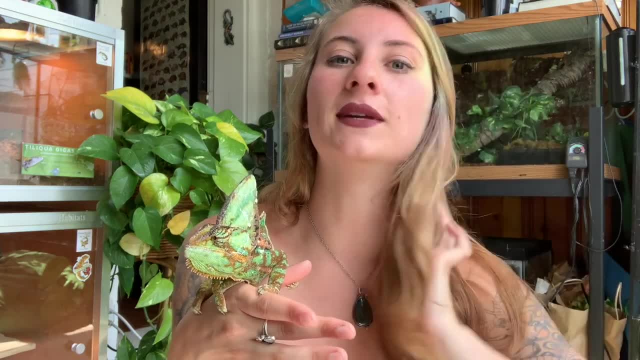 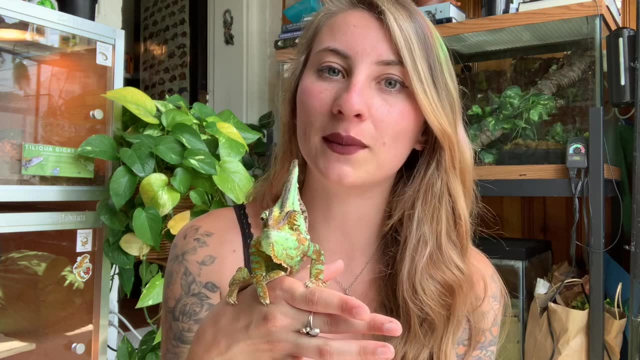 but I feel like today's video will apply to literally all chameleon species, So we're going to go ahead and cover it, because I just want to bring some awareness to the things that actually stress out chameleons, because we all know that they're highly prone to stress, and that's something. 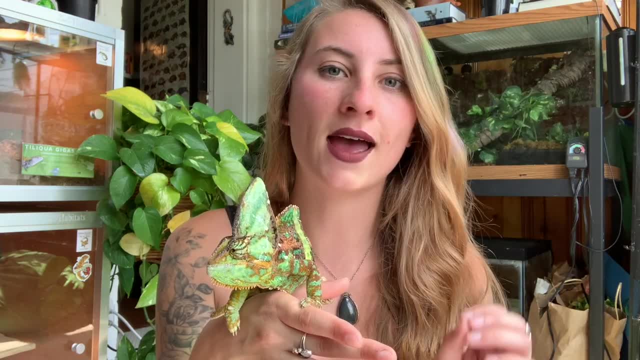 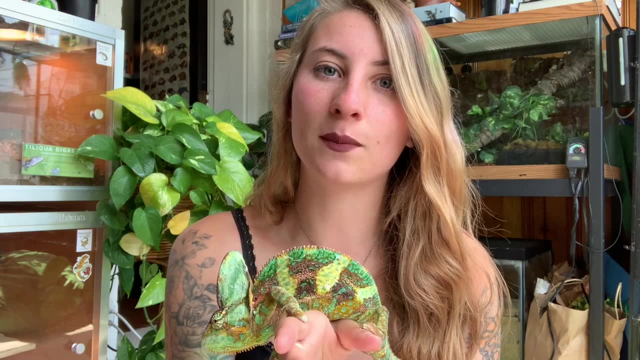 that we want to avoid. So, and I'm also not saying that every single chameleon is going to be stressed out by all of these things. They're just very common and a lot of them do get stressed out by these things. So I just want to bring some awareness today. So for number one, something. 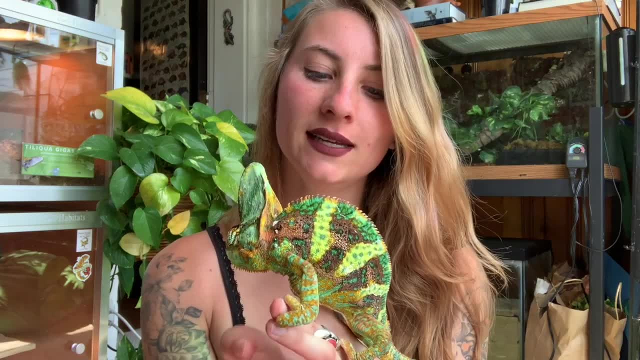 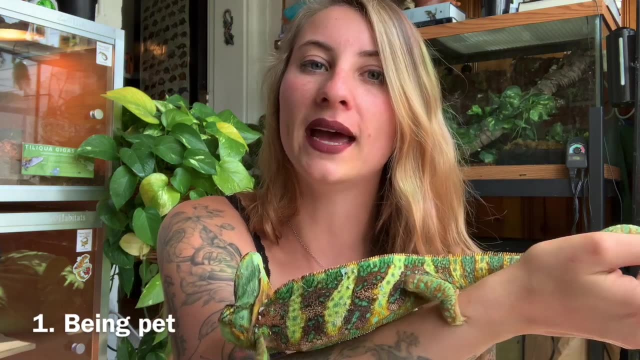 that stresses chameleons out is being pet. So chameleons are kind of strange little reptiles. They are not like a dog or a cat. They do not appreciate being stroked or pet. So that's something that I would mention avoiding for chameleons. Chameleons really aren't a type 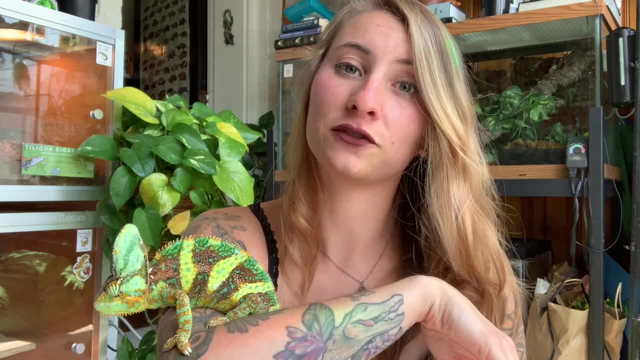 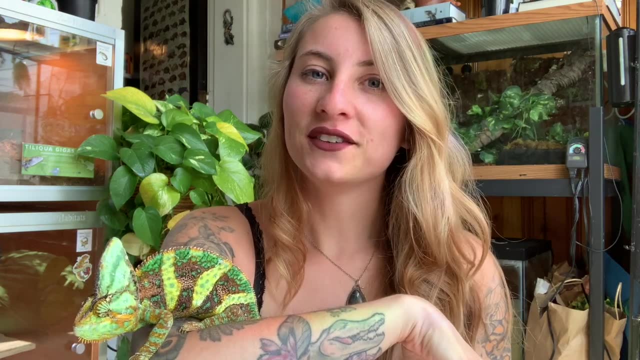 of animal that's really good for handling. I know I have Banba out for today's video, but it's because he's very tolerant and he actually wants to come out sometimes. I'm going to cover that a little bit later in the video. but one thing to do is just never pet your chameleon. 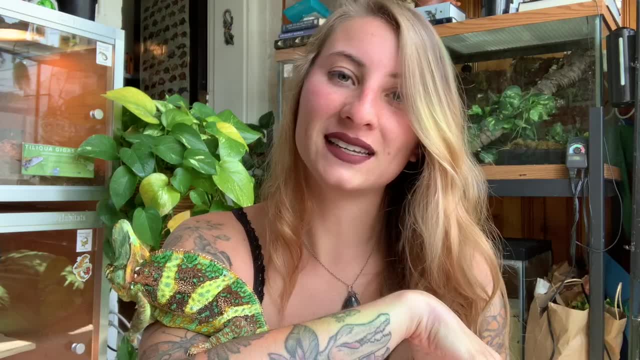 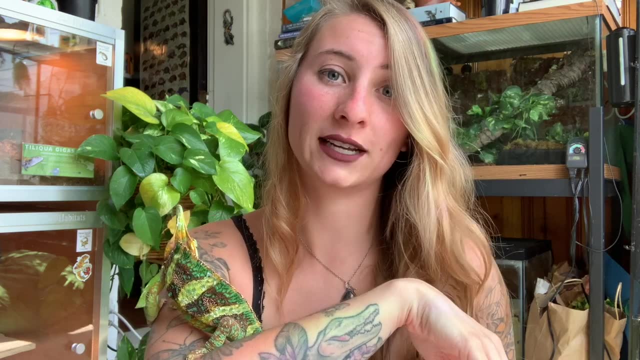 It's something that they may tolerate, but it's definitely not something that they'll ever enjoy, and they may be stressed out, even if they aren't hissing and trying to bite you. It's just something that's not comfortable or natural for them. The second thing that chameleons hate are phones, So 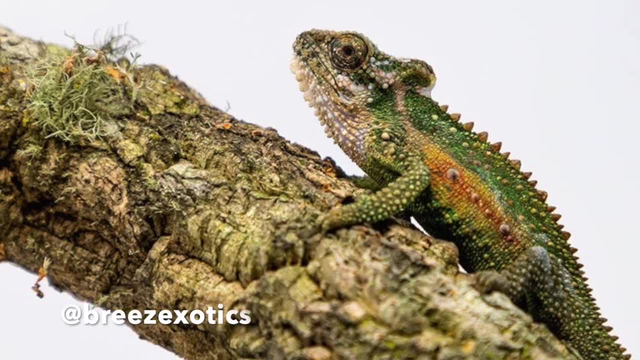 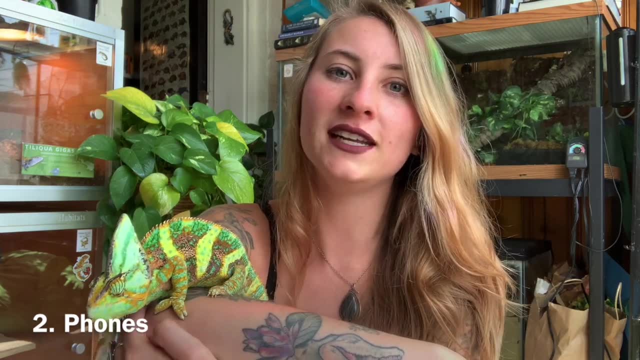 again, I'm not saying that every single chameleon hates phones, but it is very common when people are keeping chameleons as pets to take pictures of them, to take pictures of them, to take pictures of of them and videos and such. And when Banbo was a baby he absolutely hated my phone. He would hiss. 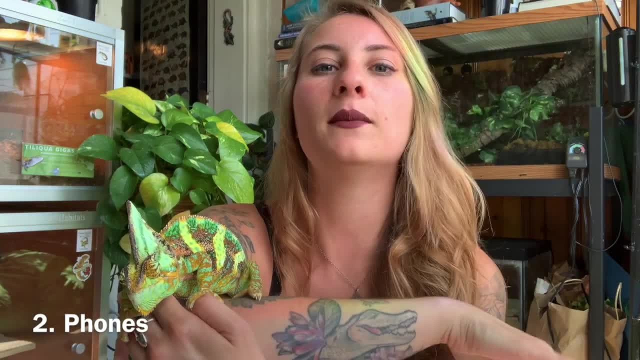 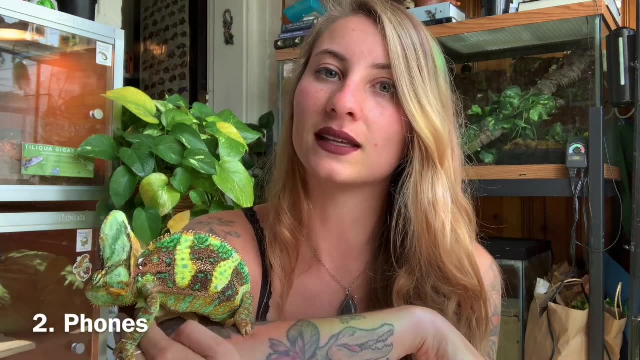 at it and get very stressed out. He would get little polka dots all over him which are an indicator of stress. So he has become way more tolerant over time and he realizes that it's not something that's a danger to him, but it is a foreign object that's very strange for these. 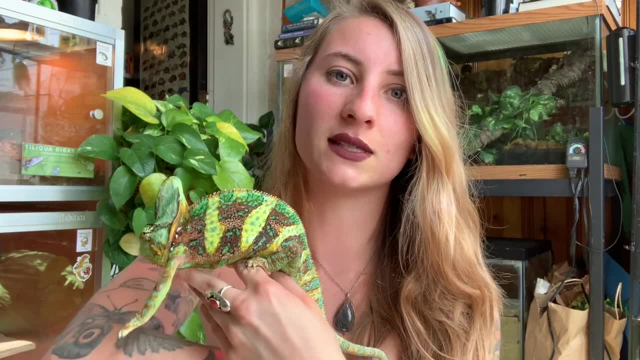 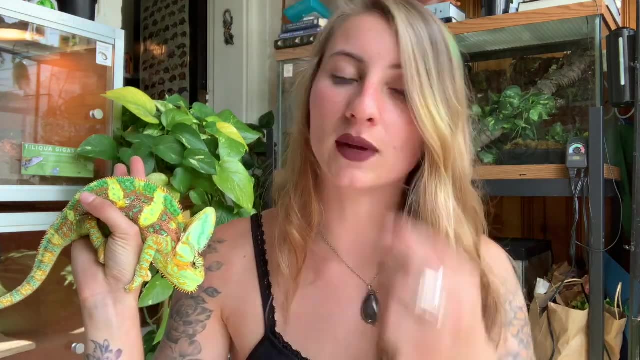 types of animals. So it makes sense that it would stress them out and cause them some fear, because they just don't know what it is. So definitely try and keep your phones away from your chameleon as much as you can, because it could be stressing them out, especially if they're hissing at you. 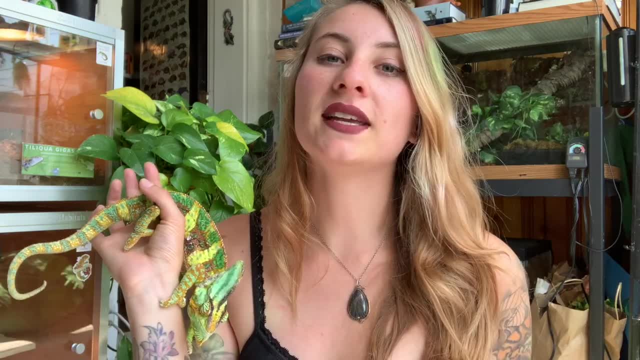 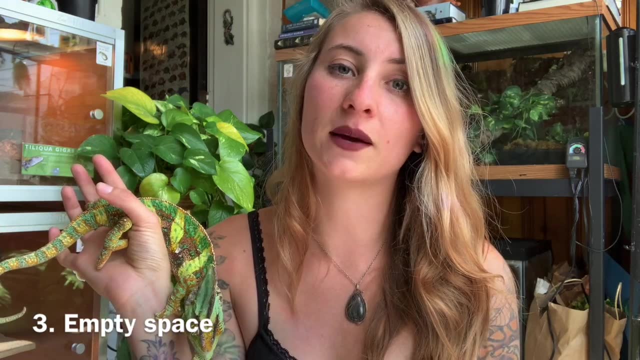 changing color and acting like they're stressed out. The third thing that chameleons hate is open space. So this may sound really random, but what I mean is, when you have a chameleon and you're setting up their enclosure, the more vines and foliage and plants that you have in the enclosure 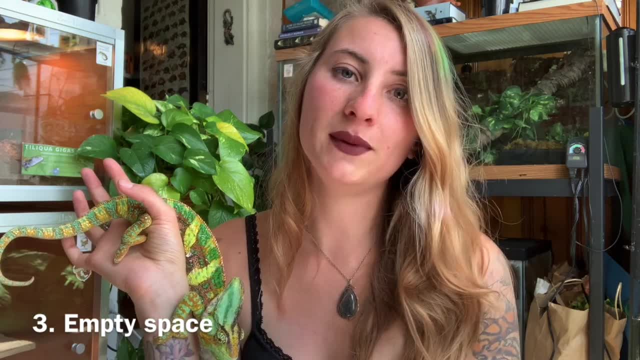 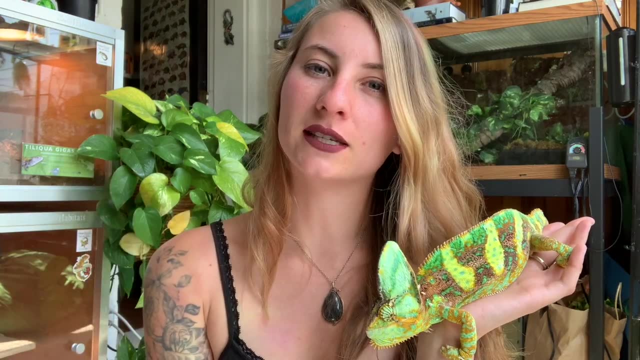 the better. If there's a lot of bare empty space, your chameleon will feel very vulnerable. They're vulnerable and exposed and it may cause stress and they may stop eating. So that's something that you'll want to avoid, because you just don't want them to be really stressed out. 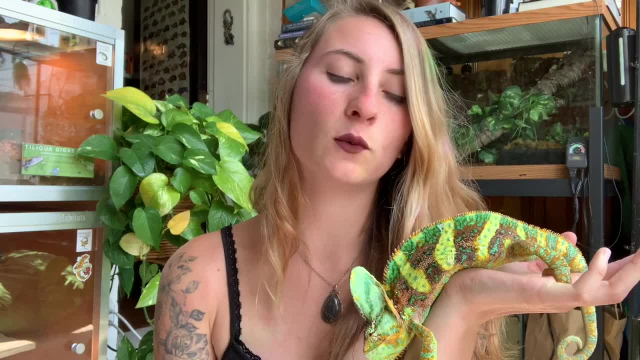 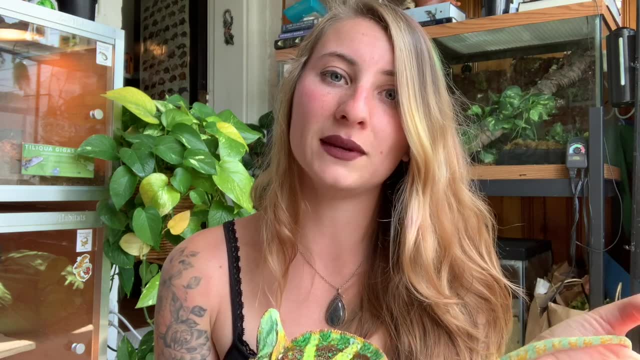 You want them to feel secure within their enclosure and then hopefully, once they feel secure, they'll start eating again, because normally that's like the number. one thing that happens is the chameleons just don't eat because they're in a new bare enclosure. So definitely fill out. 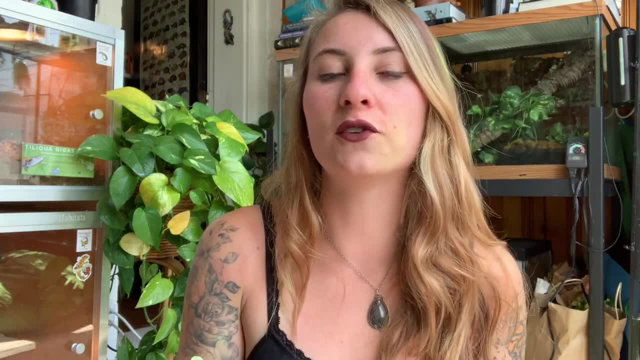 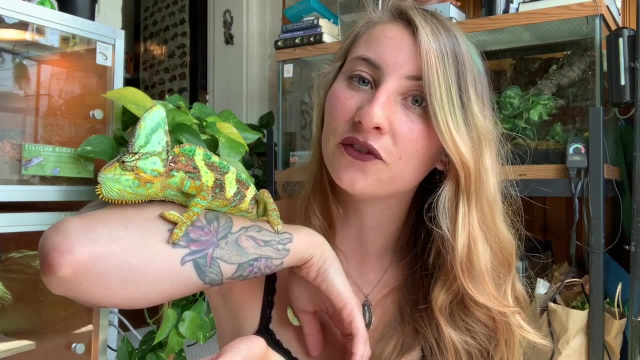 your enclosures the best that you can, because it will provide enrichment for them and they will be much happier. So Bamba is being super, super active right now. I feel like he's getting stressed out being out for the video, so I'm going to go ahead and put him back and 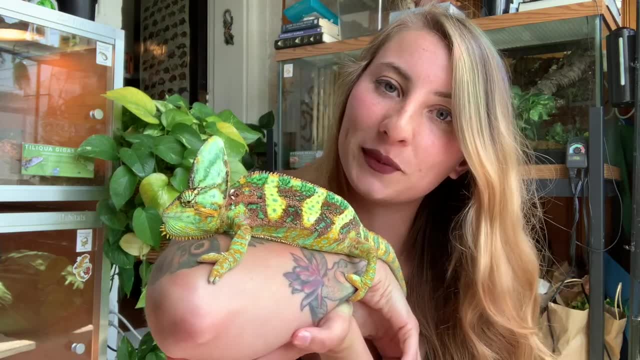 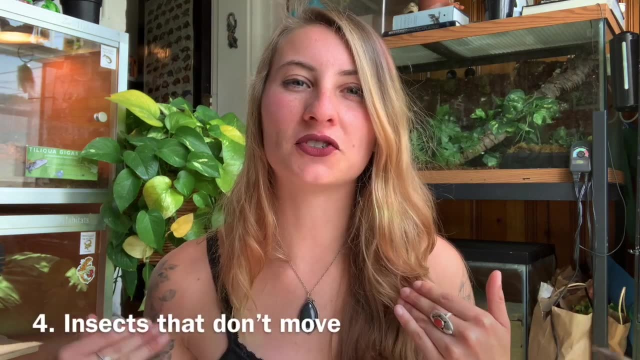 continue the video without him, but at least you guys got to see a little bit of him. So the third thing that chameleons hate is insects that don't move. So this again just sounds super weird, because people that own chameleons feed them insects, because they are insectivores. 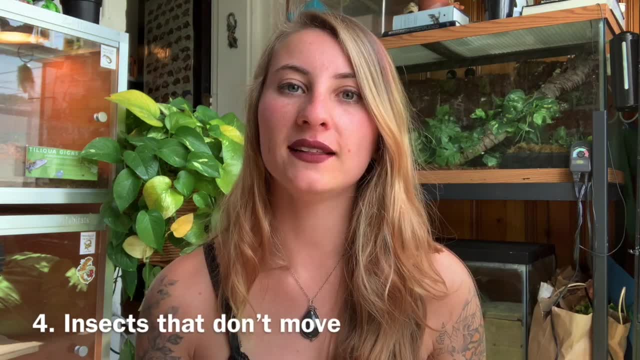 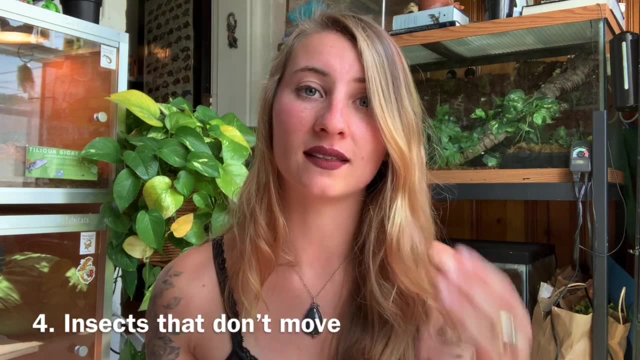 However, some people that are like new to the hobby or new to chameleons, sometimes they buy these animals and they don't like insects. They don't like the fact that they move and they can escape into the house, So they think that a way to avoid this is by getting freeze-dried insects at 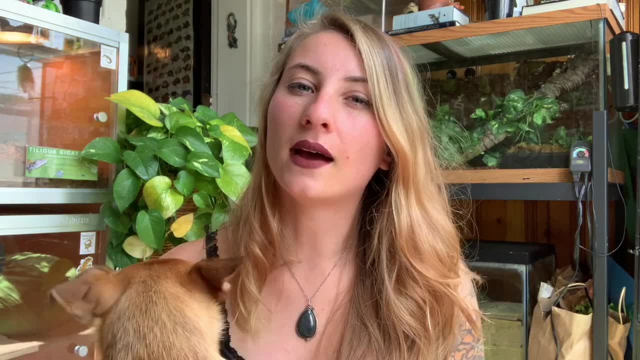 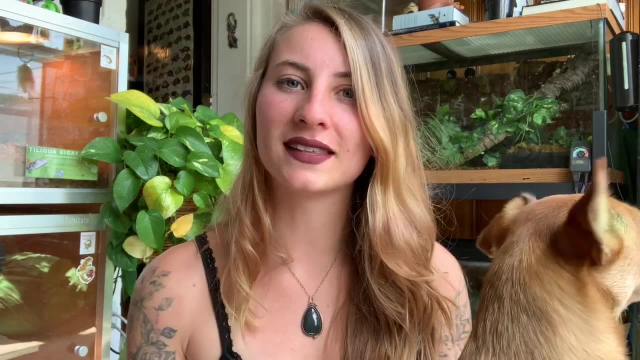 Petco or PetSmart. So this is actually a really bad option, because chameleons hunt by seeing movement. So if they see that the insect is not moving, it's not going to appeal to them at all and they're not going to have any interest. Therefore they're not going to hunt and eat it. 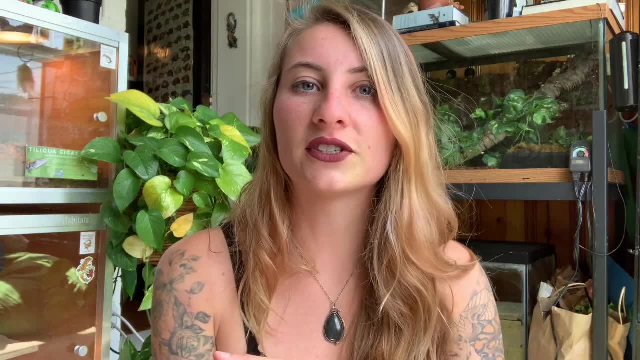 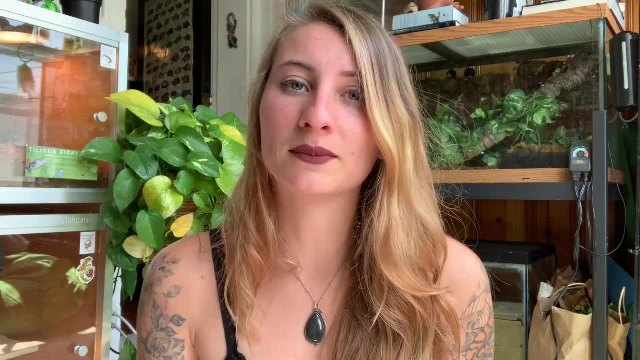 And even on the off chance it does eat it, because you shake it around or something in a cup. it just doesn't have a lot of moisture because it's dead and it's freeze-dried. So it's just not a good option because of the lack of moisture and it's also going to lack a lot of nutrients as well. 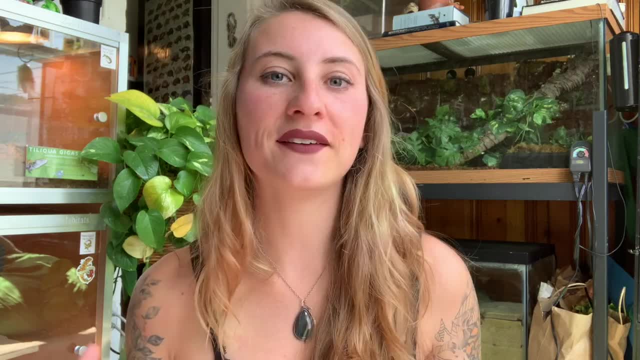 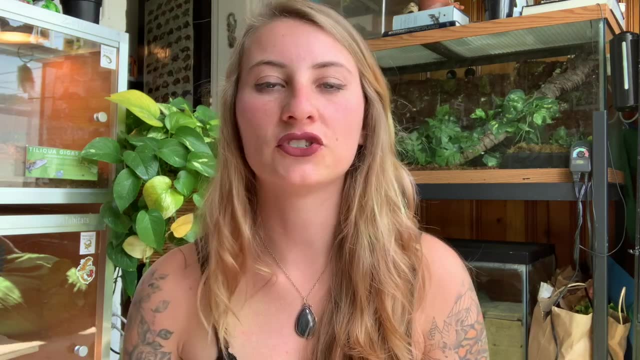 So if you're keeping a chameleon, absolutely always feed it live, healthy, gut-loaded insects, because they're going to hate an insect that is freeze-dried and not moving and or dead. It's just going to lack nutrients and it's not going to appeal to them. So if you are squeamish, 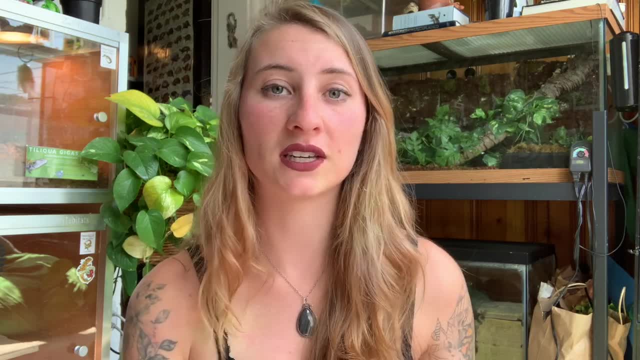 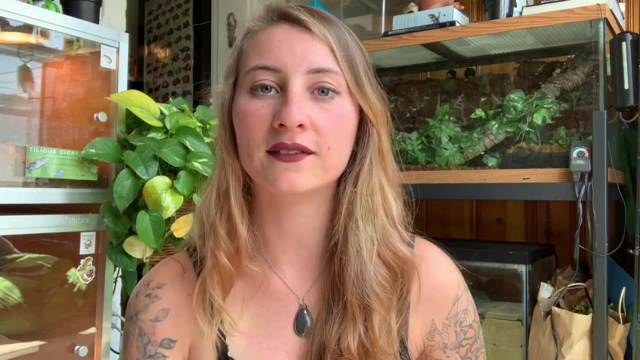 around insects and you don't want them in your house and you thought this was going to be a good alternative and you should still get a chameleon. I would advise not getting a chameleon just for that reason. You should always be giving them live insects. 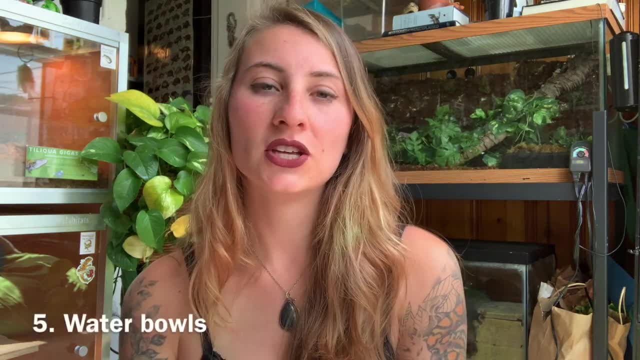 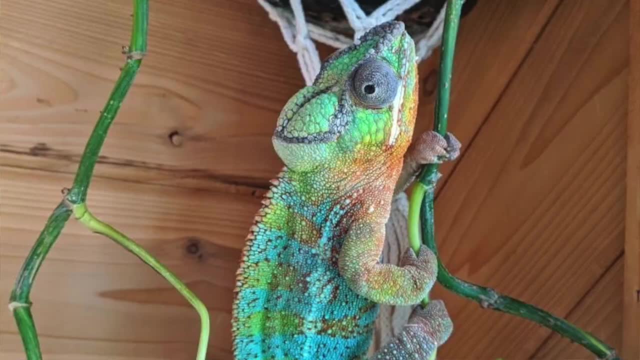 The fifth thing that chameleons hate are water bowls. So they don't particularly just hate them, but they again just don't appeal to them because of the lack of movement. Chameleons are very hypersensitive to movement around them, and that's why they hunt and that's how they 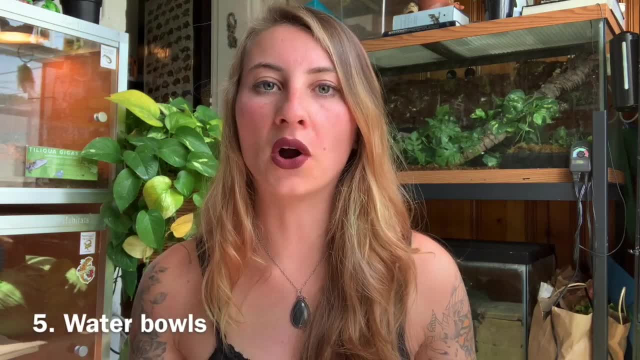 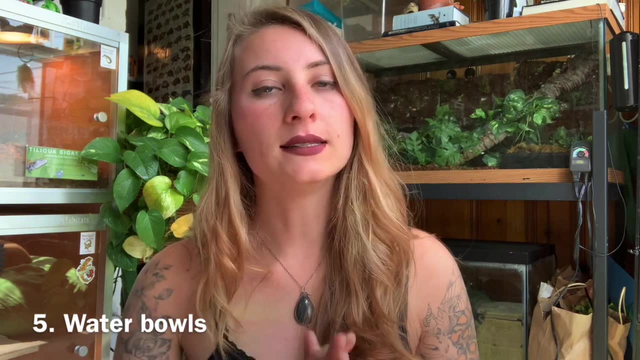 drink and hydrate themselves as well. So if you give them a water bowl with just stagnant water in it, it's not something that's going to catch their eye and they aren't going to think to just go and drink out of it In some cases. 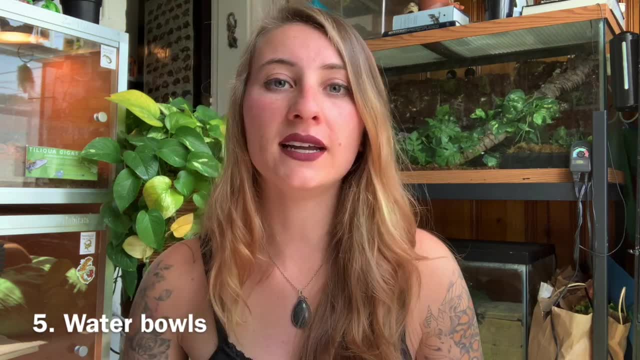 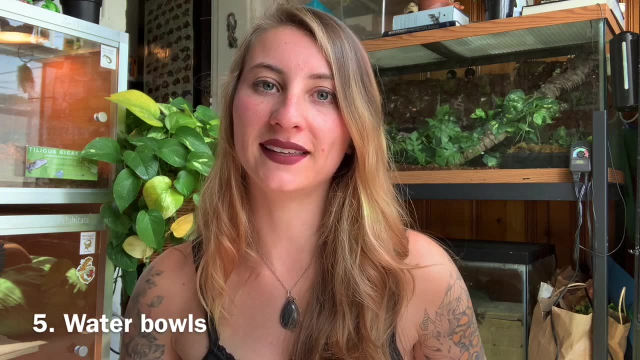 some people will say that there's does drink out of a water bowl, but it's very uncommon and it's not natural for chameleons to do that. That's why a misting system and drip system is so important for chameleons. 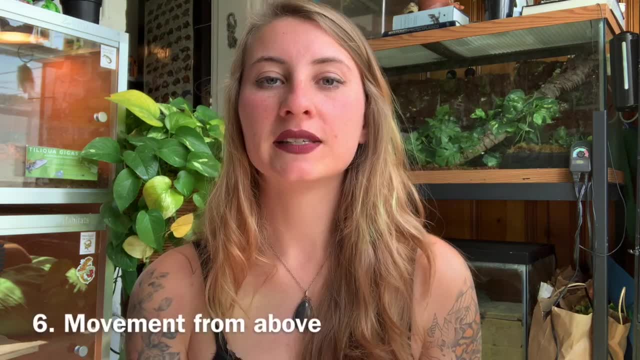 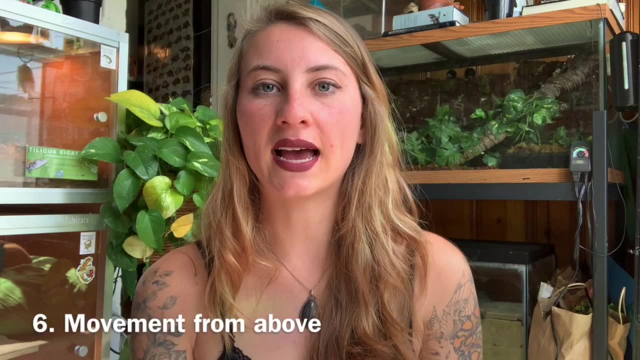 The sixth thing that chameleons hate is movement from above. So because chameleons are arboreal lizards, meaning that they live up in the trees, there are a lot of predators that are up in those trees as well, including birds that fly above them. 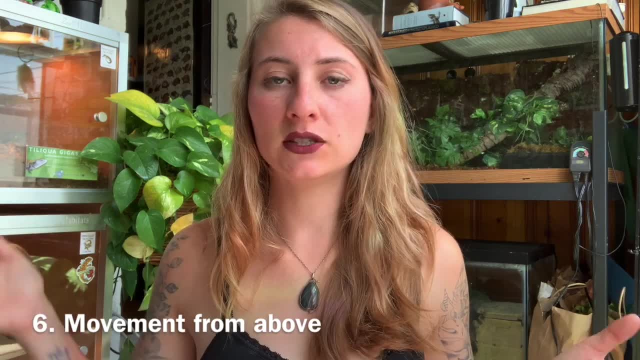 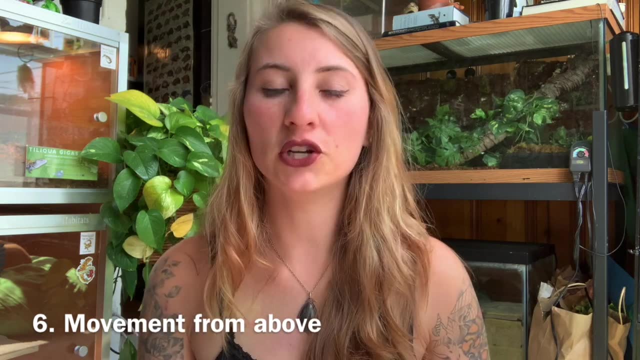 So if you are approaching them from a very high stance or reaching above them, they're going to get very upset and stressed out. They're probably going to hiss at you. They may try to bite you. They will not be very happy because they see you as a predator and they are the prey. 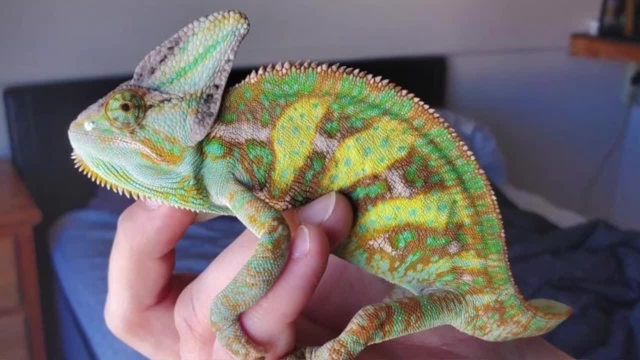 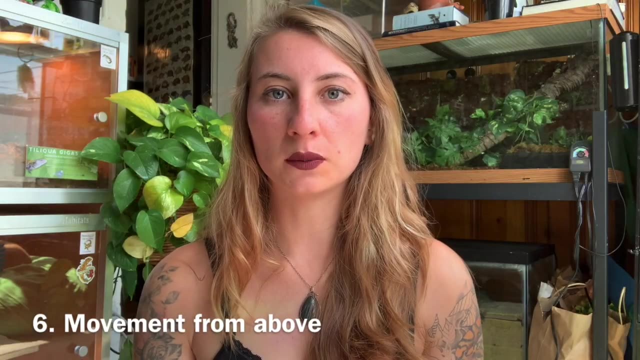 So that's something that you want to avoid. If you are trying to reach in or, like feed your chameleon or just try and take them out, the best thing to do is always reach underneath of them, Even when you're approaching, to observe them. 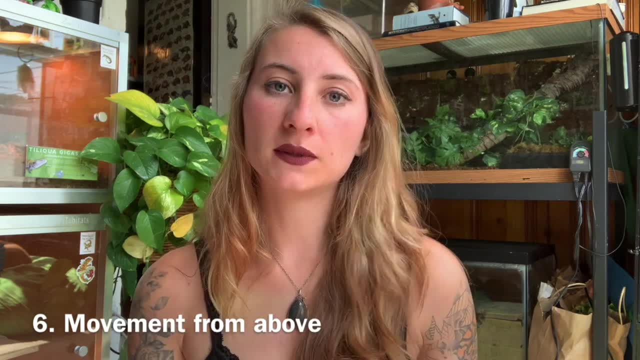 it's best to just make sure that you're lower than them. Whenever I go up to Bamba's enclosure, if I'm standing up over him, he looks at me and he's like, oh my God, like, get away from me. 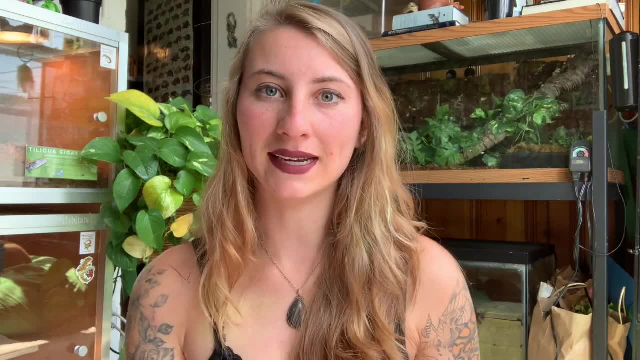 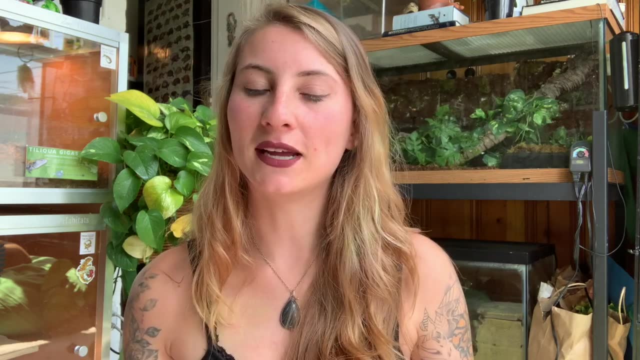 He just looks stressed out. I can tell that he's stressed by his body language, So it's definitely something to pay attention to, And because of that, whenever I approach his enclosure, I kneel down and I make sure that he is above me, because he is my king and I must worship him. 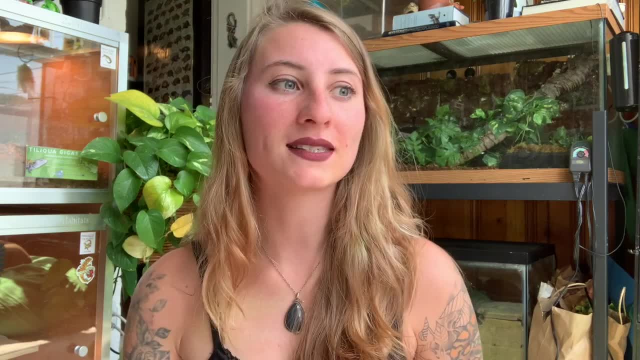 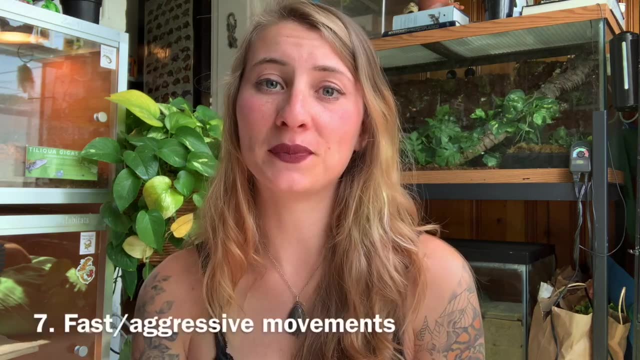 No, I'm just kidding, But literally that's how it has to be, because chameleons just get so stressed out and they want you to be under them. The seventh thing that chameleons hate are fast movements. So if you are going to reach in for your chameleon or even feed them or fix something- 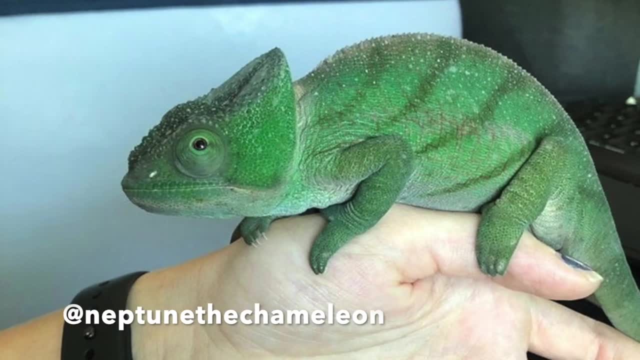 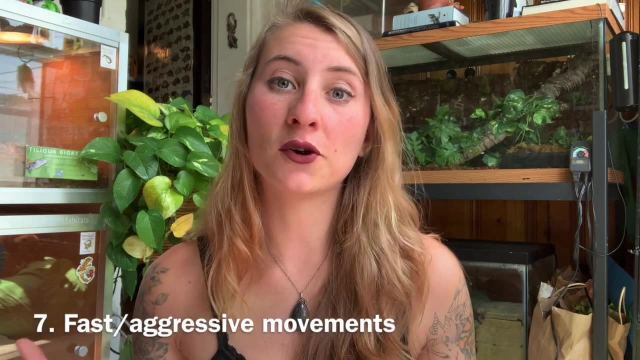 up in their enclosure. you need to do it very slowly. You cannot do jerky, fast, aggressive movements. They will get very stressed out. They are not going to like that. So whenever I go into the enclosure again, I'm underneath of him and I'm moving very slowly. 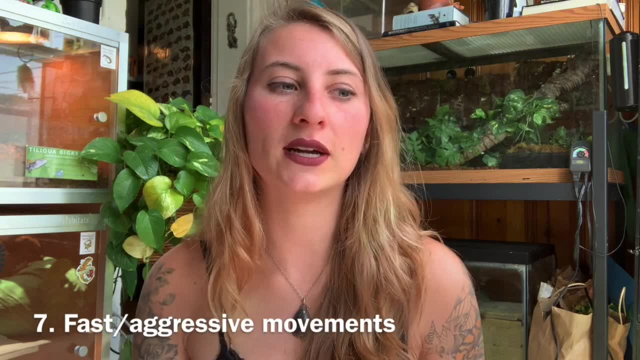 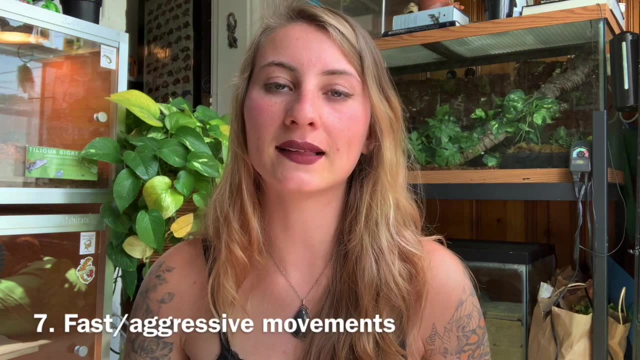 Chameleons are very slow type of animal anyway, so it's just very uncomfortable to them If you were to be moving super fast and aggressively toward them and they're most likely going to be hissing and extremely stressed out. So it's best to just be very 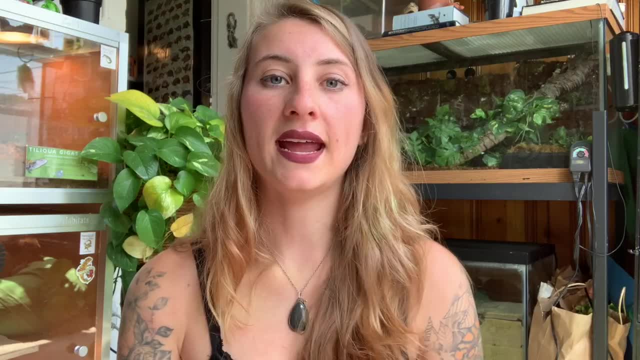 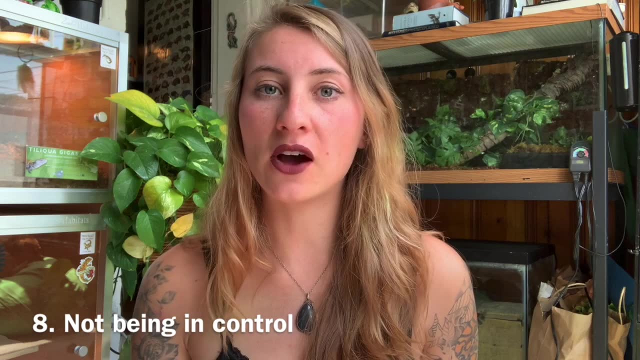 very calm and Zen when approaching a chameleon. The eighth thing that chameleons hate is not being in control. So this comes with handling and taking them out and making them do things that they don't want to do. It's kind of hard to talk about things like this. 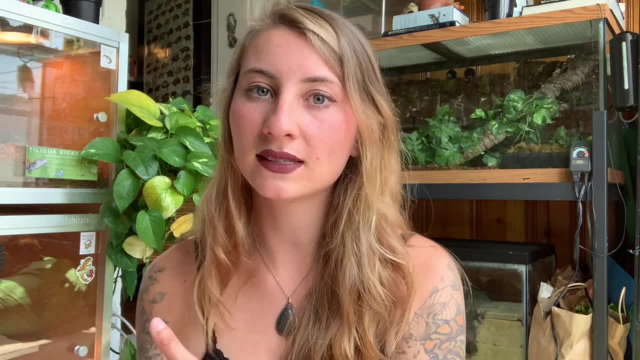 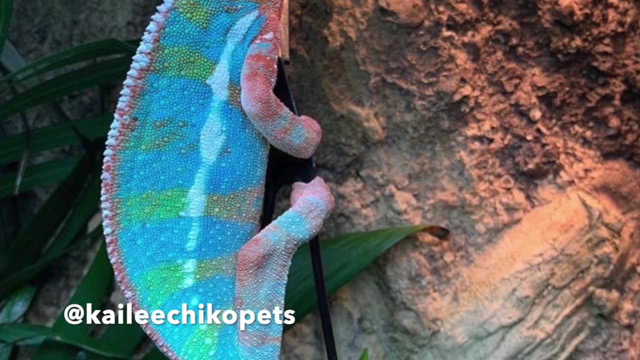 because people think that I'm anthropomorphizing by saying that they want something or they don't want something. However, with chameleons, it is very easy to understand their body language. with chameleons, They let you know when they don't like something. 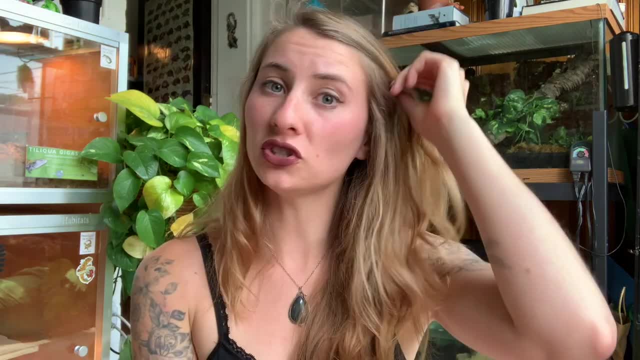 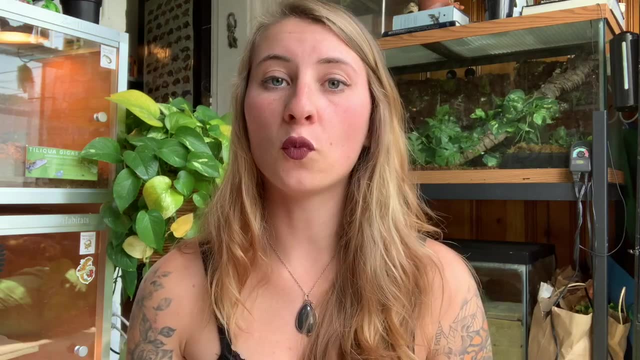 They will hiss, They will be very aggressive toward you, especially veiled chameleons in particular, but it is something to be aware of and respect that boundary. If they don't want to come out to you, they aren't going to climb out onto your arm. 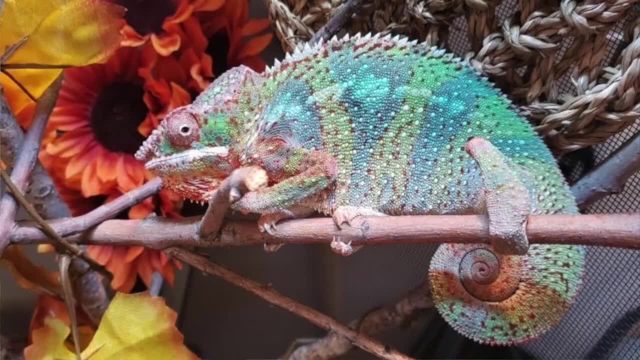 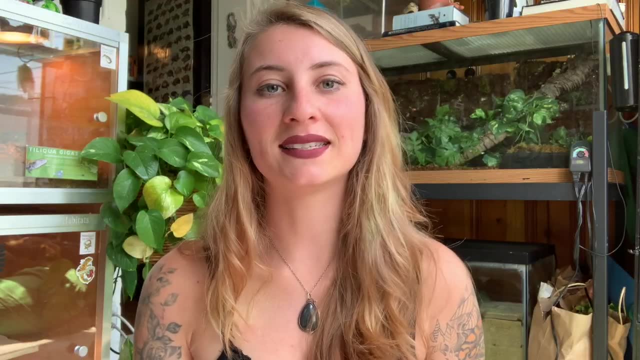 then it's best to just leave them alone. It's good to let them always be in control of the situation. That way they can choose what they want and don't want to do. That way you're not pushing them too hard, Like today. Banbo was okay coming out. 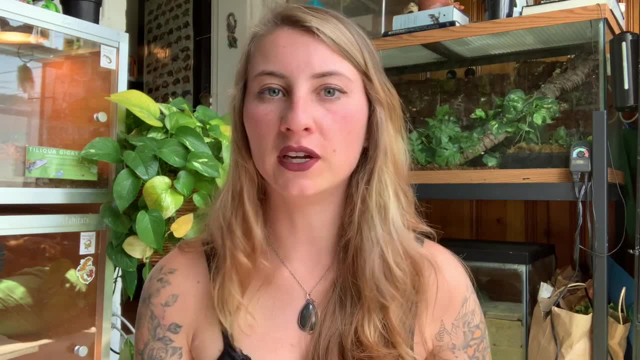 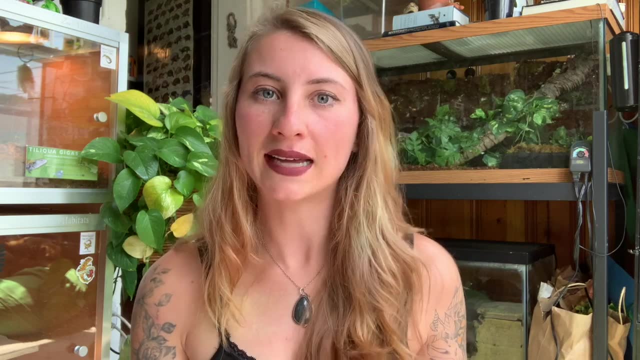 He wanted to come out, but then he just seems stressed out. He was moving all over the place And just did not seem very relaxed. So because of that I decided to put him back and now he's calming down, Now that he's back in his enclosure. 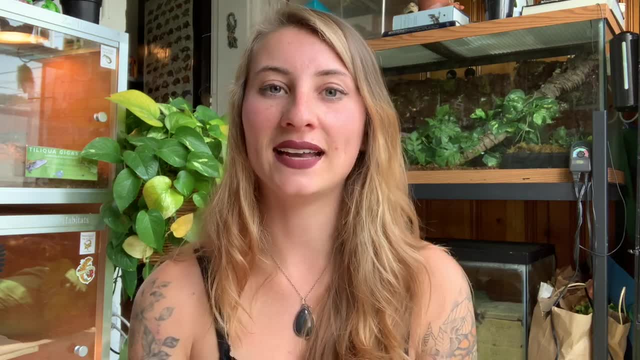 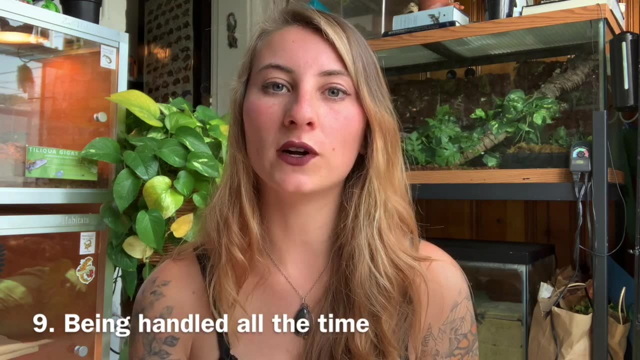 which leads me to number nine things that chameleon hate and that is being handled all of the time. So chameleons are more of like a look, don't touch type of animal. Some of them will go up to the door like Banba. 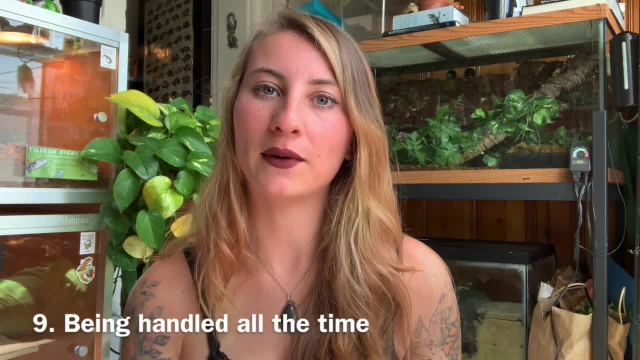 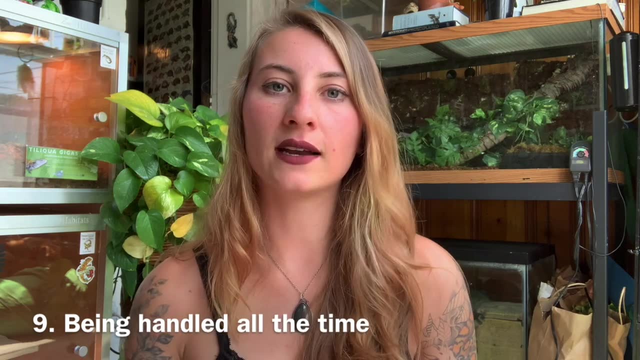 and, like he literally goes by the door, waits for me to open it. That way he can crawl out onto me, which is why it makes it seem like he wants to come out because of that action, Whereas a lot of them will just not want that. 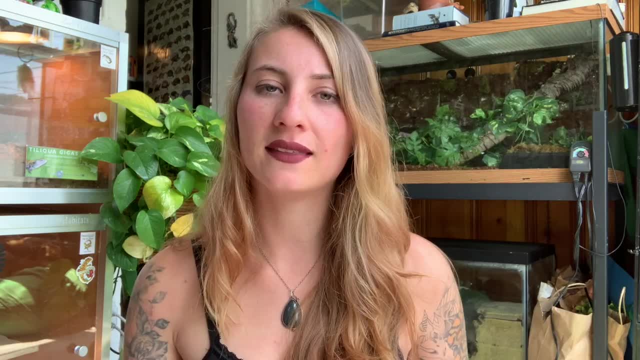 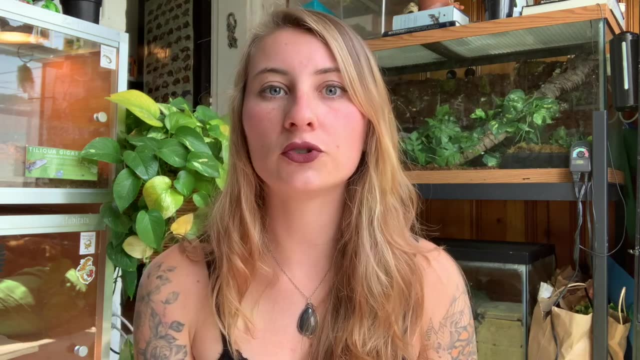 They will not crawl out onto you. They just kind of do their own thing and that's completely fine. But if you have to take your chameleon out, whether they want to come out, or you need to clean their enclosure, or whatever the case may be, 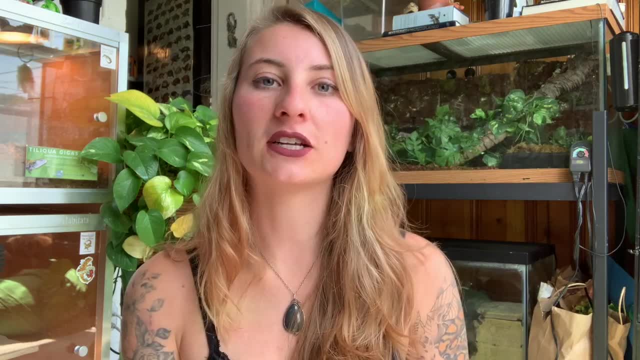 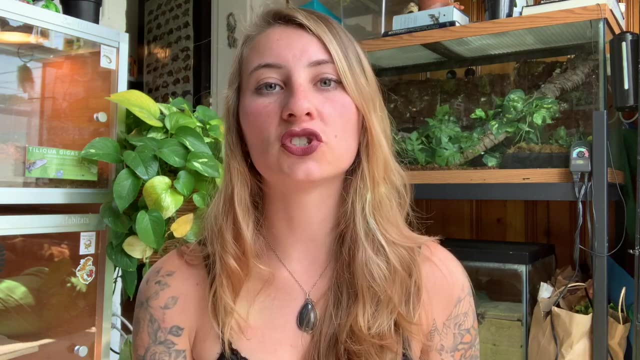 it is important to keep handling sessions very short, especially if they're getting stressed out, like what happened earlier with Banba. I could tell he was getting stressed out and that's why I put him back. So it's just very important to respect those boundaries that they have. 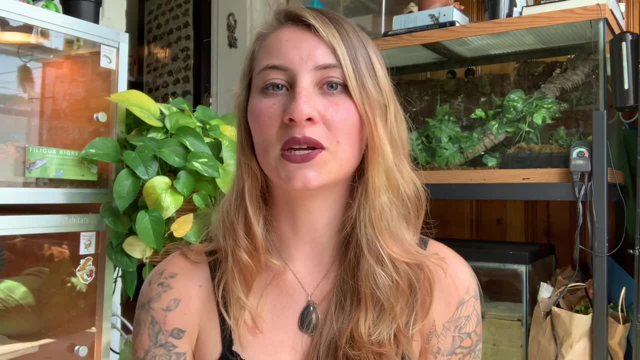 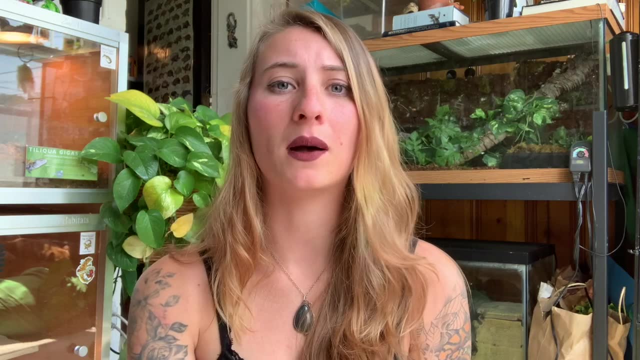 and not push them too hard. I would also recommend not taking chameleons out and like for hours at a time, or like visiting a group of people and showing them off going to public places. That's absolutely going to be way too much stimulation for a chameleon. 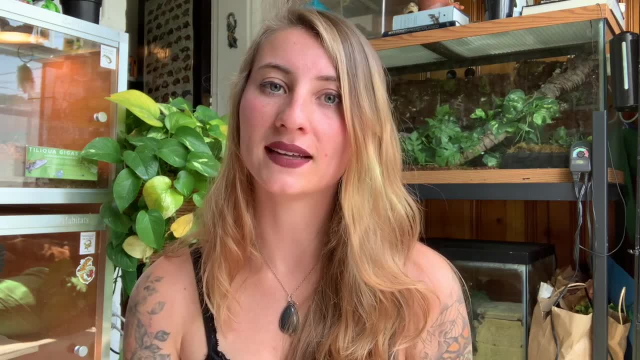 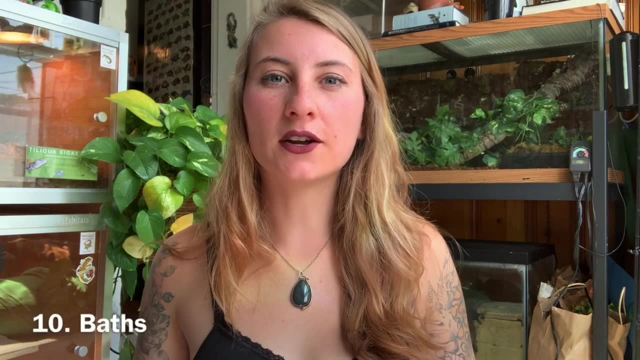 It's going to be really stressful on them, So it's best to avoid that. And for number 10,, the last thing that I have for today that chameleons hate are baths, So baths are not a requirement for chameleons. 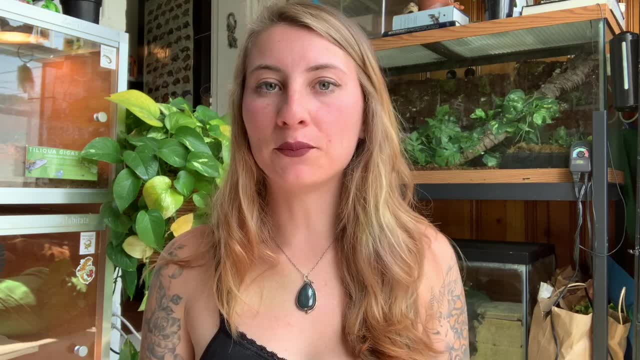 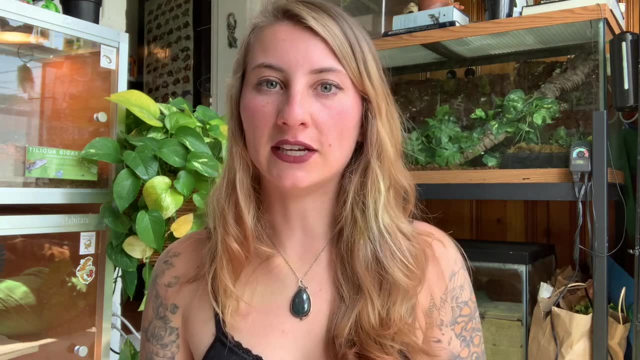 when you're keeping them as pets whatsoever. The only reason I'm bringing this up is because it was a learning experience for me, because when I first got my chameleon, I was not aware that they are dry shedders. I thought that he needed help. and I should bathe him to try and get the shed off. Obviously, it wasn't sticking him in like a tub of water. Chameleons do not swim. What I would do for this is hold him in my hand and bring him to a sink with warm water. 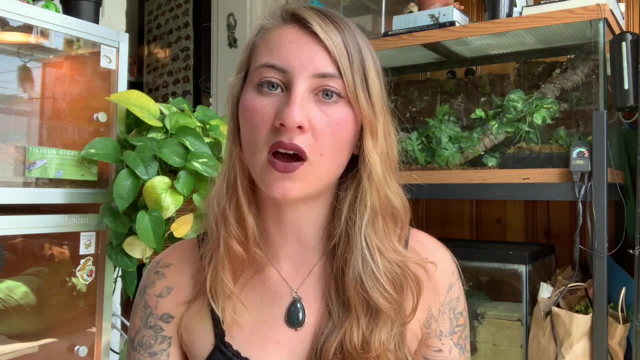 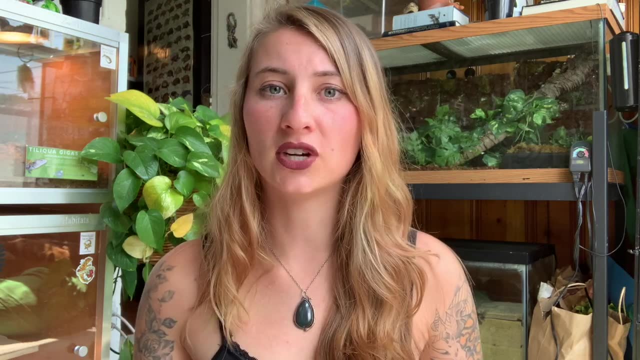 and just let it rinse on him lightly, just to try and get the shed off of him, and I would try to like massage it off of him. I absolutely hated this. It was very stressful for him. He was constantly trying to get away, constantly trying to grab the water. 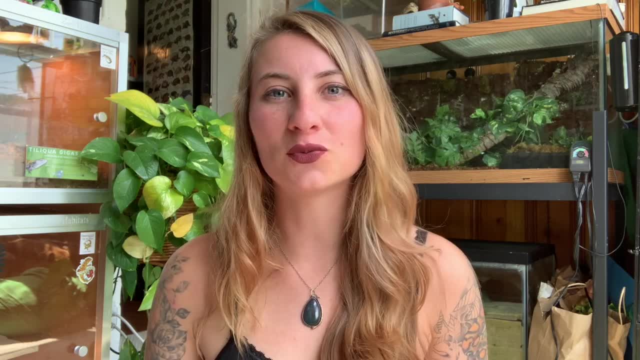 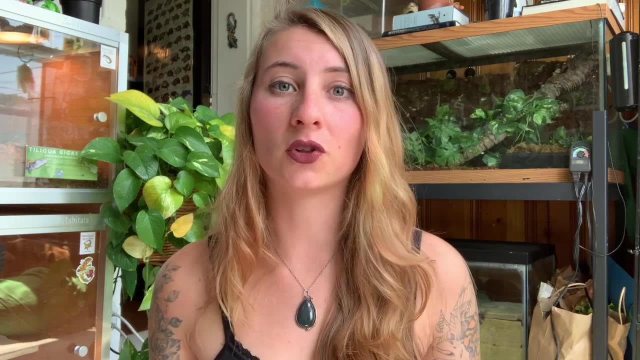 which is something that, like everyone thinks is really cute, but it's actually just really stressful because they're trying so hard to grip something that they can't grip because it's water. So the whole experience was a learning experience for me. It wasn't necessary for him, number one.